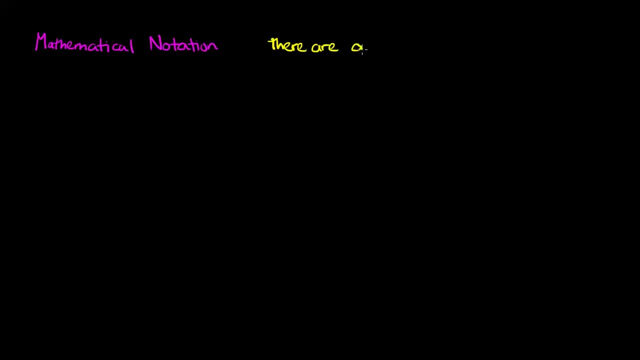 Think about this example: If I write there are only four ways, or if I write the number of ways is only four, The second way could be very misleading, because four with an exclamation means four. factorial, That's four times three times two times one. So notation is important. 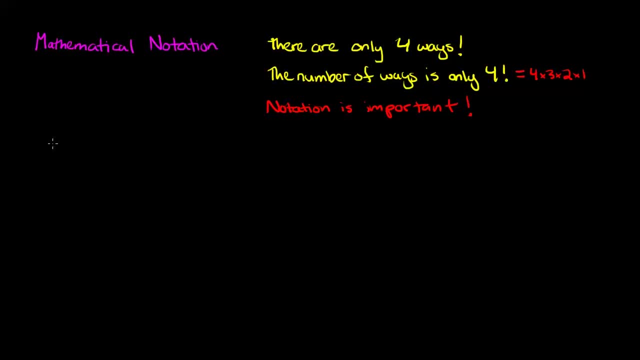 In this video I'd like to discuss some important notation that you're sure to come across in discrete mathematics and graph theory. Some basic counting notation- since I've already brought it up, is n factorial. Now, n factorial is equal to one if n is zero, and otherwise n factorial is. 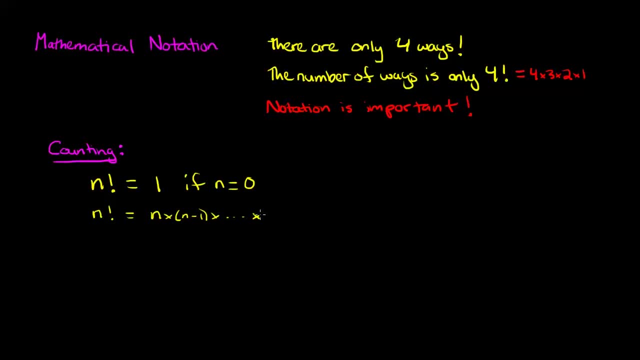 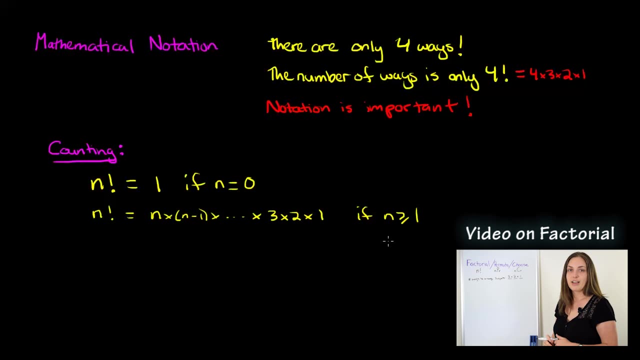 equal to n times four. So if n is zero, then n factorial is equal to one. if n is zero, n factorial is equal to n times n minus one, times n minus two, and keep going until you get to three times two times one, and that's if n is at least one. n factorial counts the number of ways. 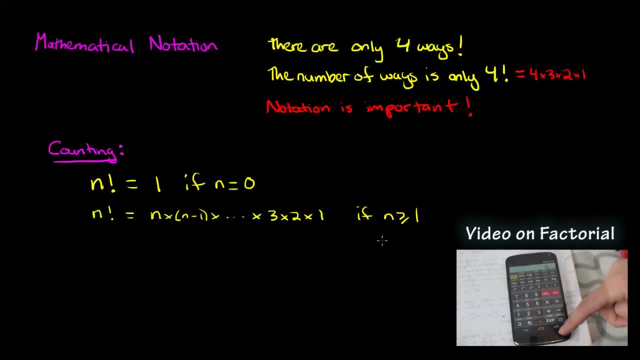 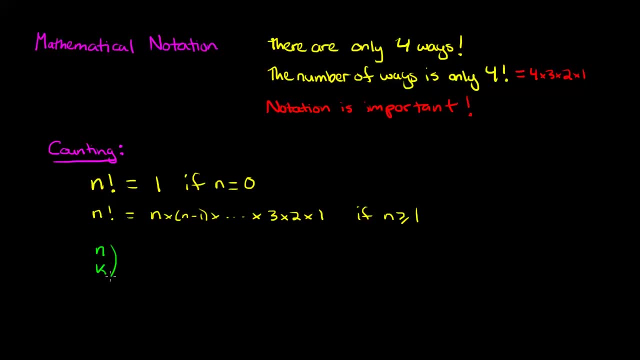 to arrange n distinct objects. So notice that if you have zero objects, there's one way to arrange them. Do nothing. Related to this is the binomial coefficient n above k. This is also written as nck sometimes, and it's equal to n factorial divided by n minus k factorial times k factorial. 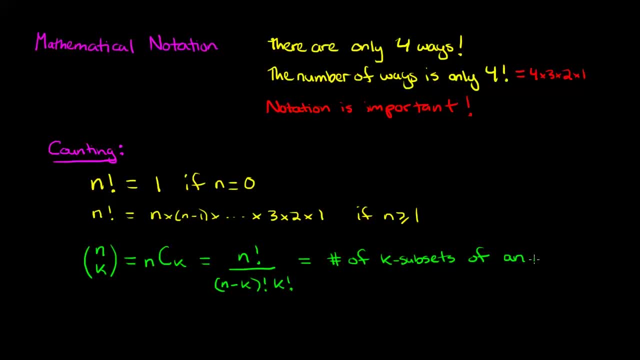 And this is the number of ways to arrange n distinct objects. So notice that if you have zero objects, this is counting the number of k subsets of an n set. So here we think of n as a non-negative integer and k also as a non-negative integer which is less than or equal to n. Now, since I've 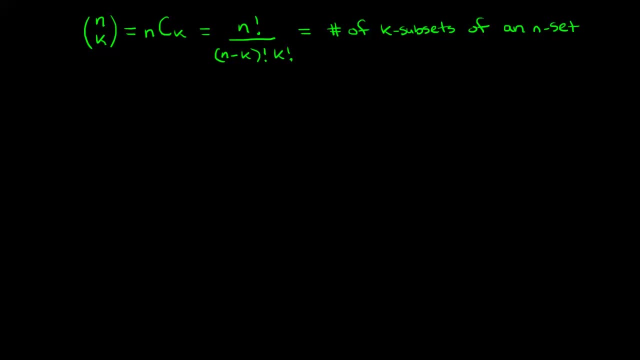 brought up the idea of sets. let's take a look at some key notation that has to do with sets. We write down our set as elements written inside of squiggly brackets. For example, one, two and three might be inside of my set. I may also have a set that has one, two all the way up to 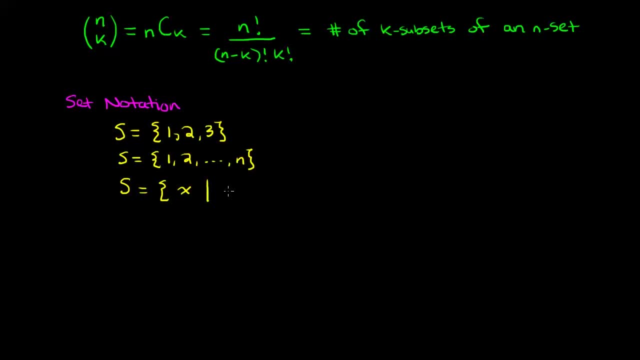 some number n. So if I have a set that has one, two, all the way up to some number n, I may even choose to write this as all the values of x, such that x is between one and n, And this is equivalent to the one that I just wrote before. The key thing is that in a set, 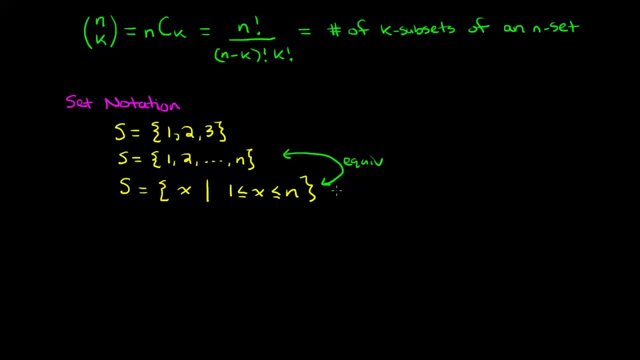 we don't have any repeated elements, So we wouldn't write one, one, two, three, we would just write one, two, three. We can think of a set as a basket of things and we don't have any repetition of those. 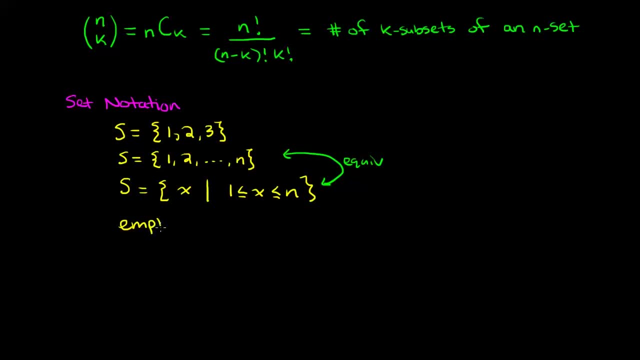 things. But we may even have an empty basket. So that's like the empty set, which is just denoted by empty braces, And it also has a set that has one, two, all the way up to some number n. So we 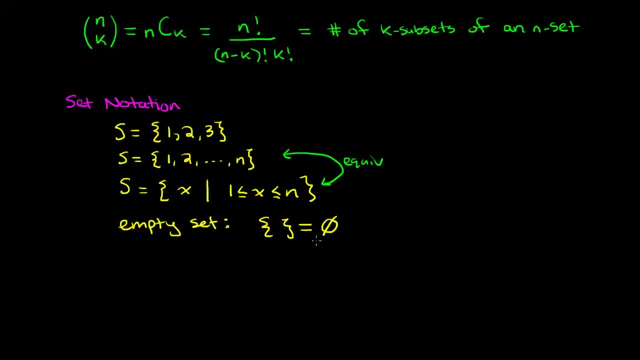 special notation written like this: Now, keep in mind that our set doesn't have to just contain numbers as its elements. it could contain vertices, or strings of letters or anything like that- basically, anything that you want to be talking about. So let's take a look at an example of a. 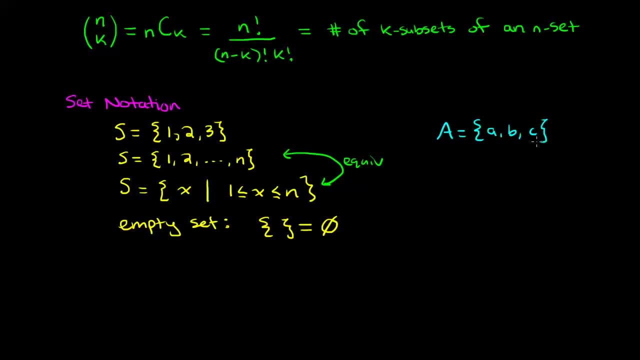 set, capital A, which has a, b and c as its elements, then we can use this notation a in capital A to mean that little a is an element of capital A. we can say that four is not an element of the set a. So that's the notation when you're dealing with an element inside of a set. But you 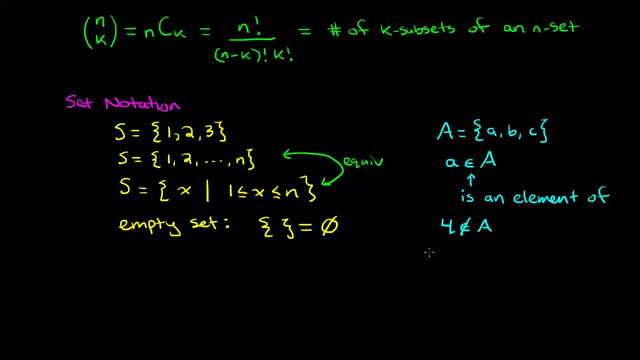 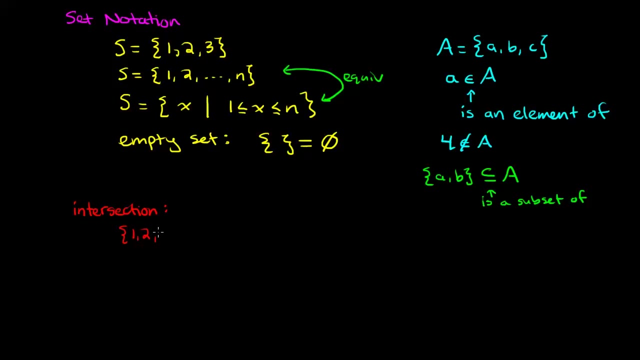 can also talk about a set which is itself contained inside of a bigger set. So if I look at the set a b, that's contained in a, so I use this notation to show that it's a subset of a. we can also take the intersection of two sets. So here's an example: the set 123 intersect with one two. 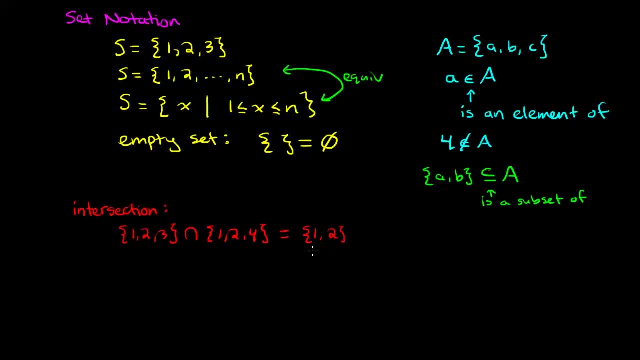 and four. the intersection is one and two because it's the place where one, two and three agrees with one, two and four. So to be an element in the intersection you have to belong to both of the sets, the union of two sets. let's take a look at an example: one, two and three. 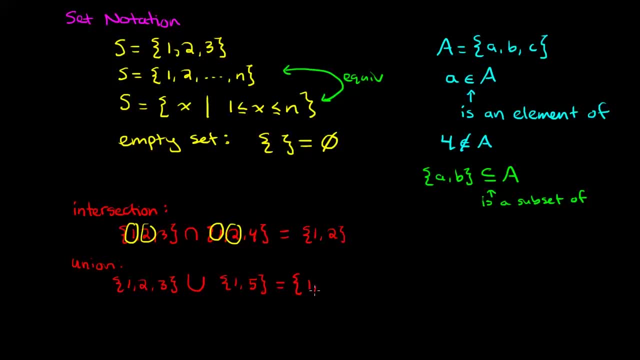 union with one. five is one, two, three and five. Here we take any element that's in either one of the sets or in both sets. If we want to take a look at a picture that represents these ideas, we can think of this set A as the purple set and the set B as the blue set. 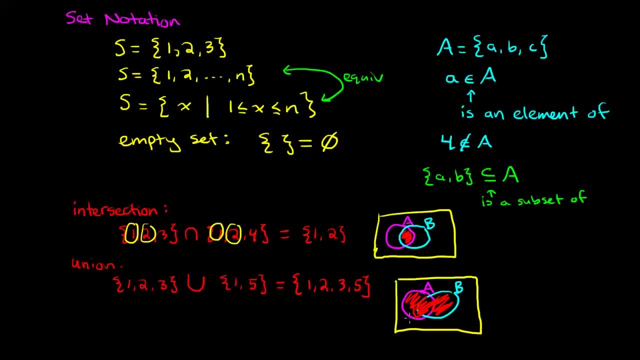 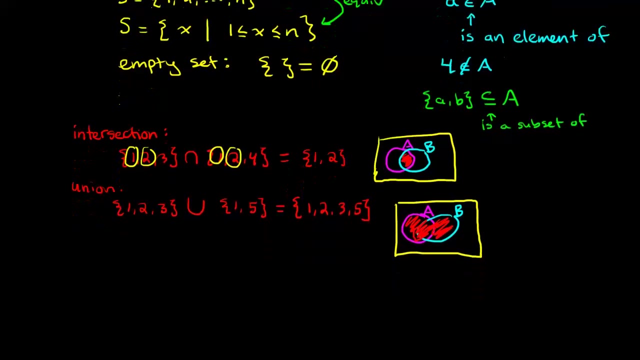 the intersection is whatever they share and the union. if we have again A and B, the union is any element that's in A or B or both, this whole piece. it turns out that we can actually generalize and take lots of unions of different sets And we have a new notation for that as well. Let's say that. 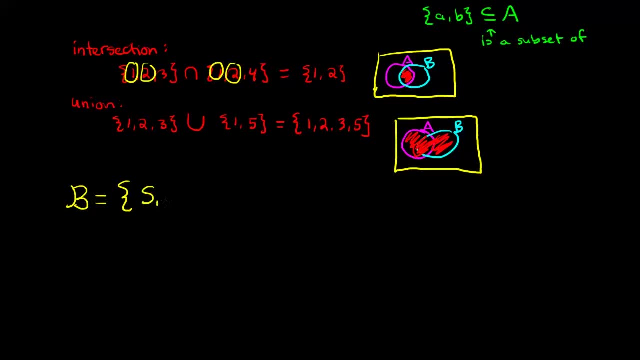 this curly B is equal to a set which has in it s1, s2 up to sk, where in fact each of these si is a set for i equal 1 up to k. Then we might be interested in taking the union of all. 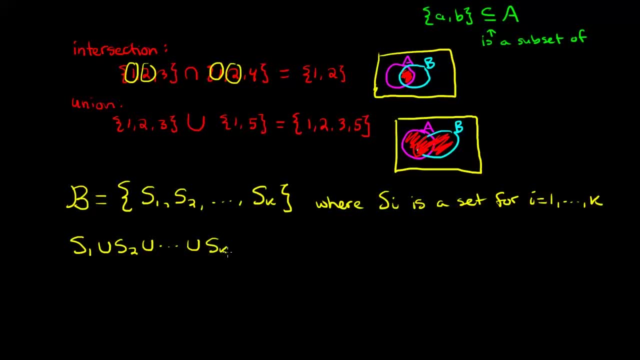 of them: s1 union, s2 union, all the way up to sk, and our new notation for this is a really big union, and underneath that we can write s as an element of the set B, and then we write s, the thing we're going to take unions of Now. notice here: 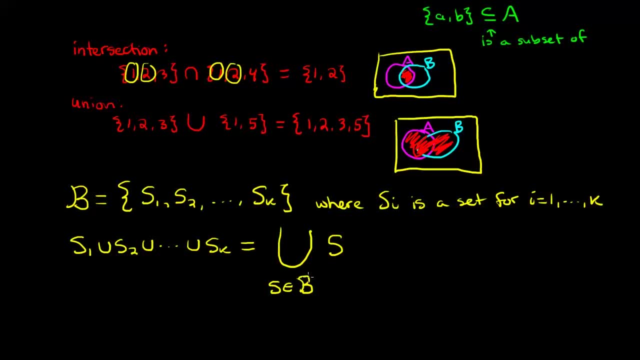 that we can write s is an element of this set, even though s itself is a set. The reason is because this curly B is a set which has as elements sets, So in this sense s is an element of B. This type of notation is really useful if you. 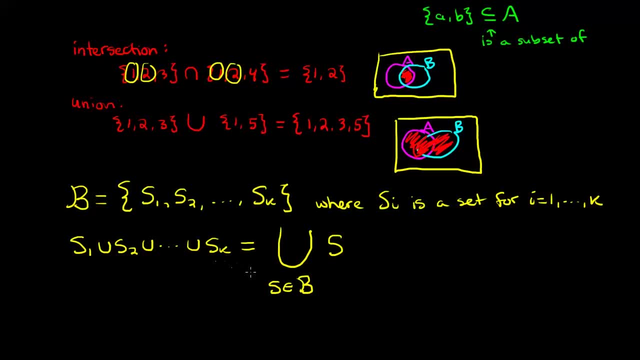 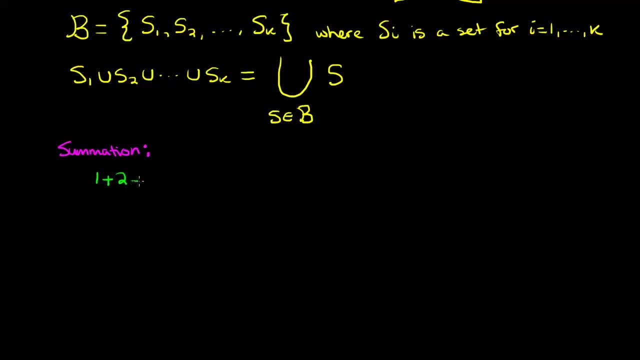 don't want to write out all of the pieces of the different unions. This is familiar if you've seen the summation notation, so let's take a look at that now. If we have the sum 1 plus 2 plus 3 plus 4 plus 5, we could also write this: 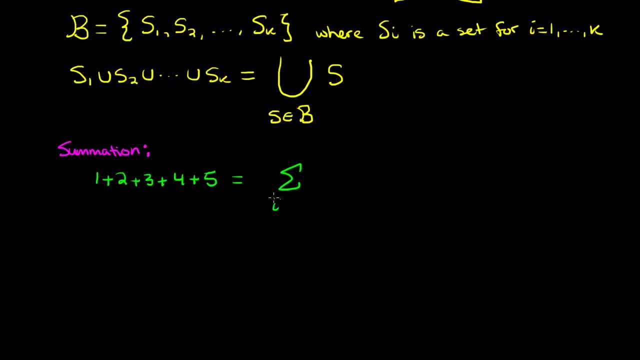 using this capital Sigma below here. So if we have the sum 1 plus 2 plus 3 plus 4 plus 5, we could also write this using this capital Sigma: below your we write i equals 1, and on the top we write 5 of i. What this means is we're. 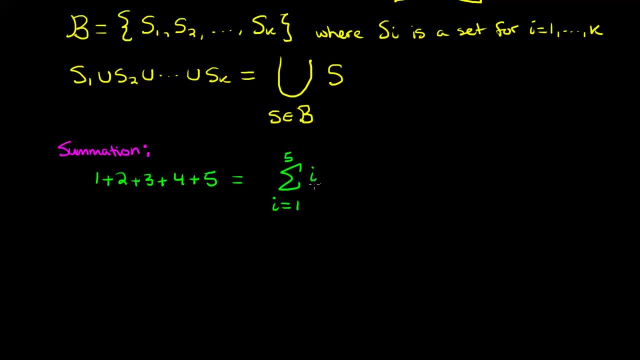 summing up all these values of i, starting at i equals 1 and going on and on until we get to i equals 5.. That's our stopping place. We can do things that are more general, like if we were looking at 3 squared plus 4 squared, all the way up. 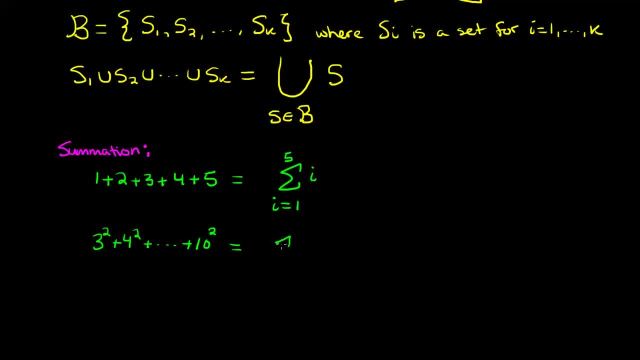 to 10 squared, then you would say the sum from and you don't have to use i let's use n equal 3 up to 10 of n squared, and you should be able to see that plugging in values of n from 3 up to 10 gives you exactly the sum you're. 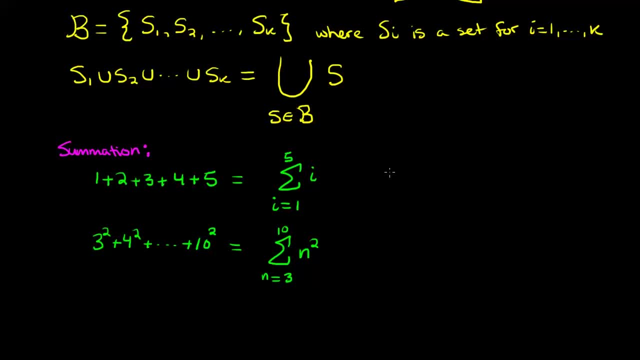 looking for. This is very convenient because you can be very much more general. like this: You could say something like 2 plus 4 plus 6, up to 22, and that can be written as the sum from i equals 2, but not just from i equals 2. 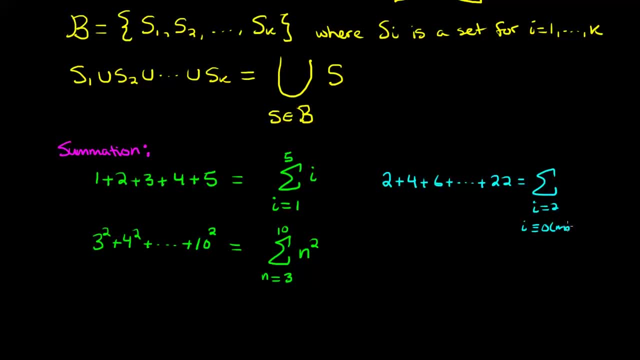 because you don't want to use the number 3. so you could say: from i equals 2 where i is 0 mod 2, in other words, where i is even up to 22.. In other words, you can write extra conditions in the bottom of the sum if required. Sometimes we even 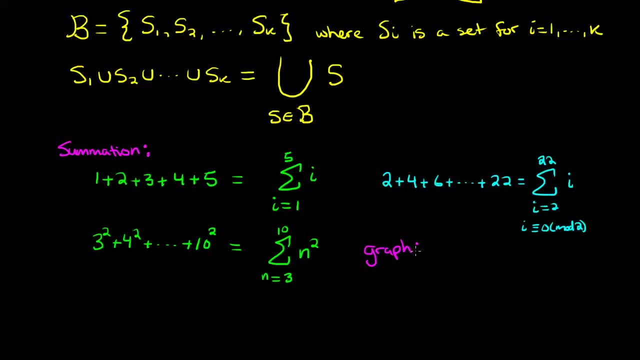 want to use a summation notation with sets. so here, if I have a graph which has vertices x, y and z, I may be interested in the sum for all vertices in my vertex set and I want to sum up all the degrees. So that would be equal to in this case, 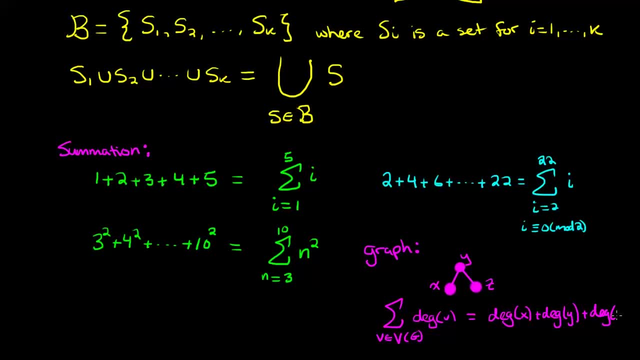 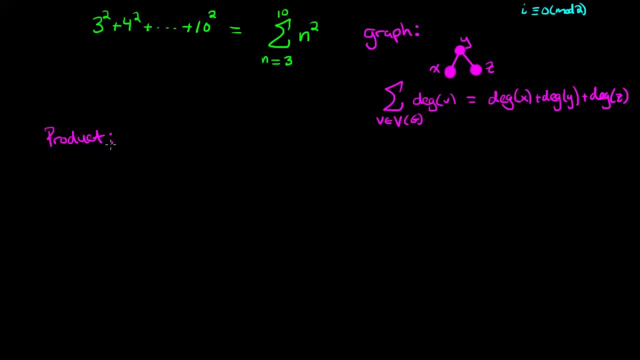 the degree of x plus the degree of y plus the degree of z. and if you have a graph with many vertices, it's very convenient to use summation notation and you can do a similar thing for a product. So if you have this sort of capital pi with of n squared minus 1 for 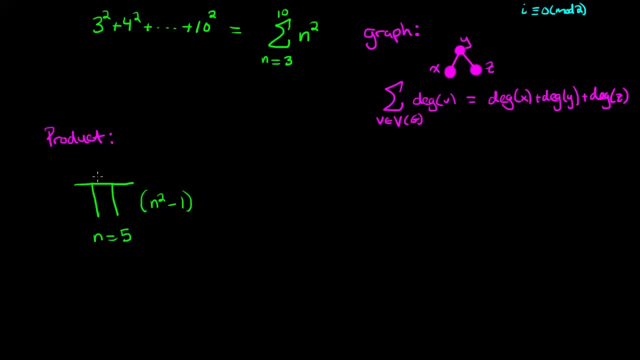 n equal to say 5, up to capital N, this would be equal to the product 5 squared minus 1 times 6 squared minus 1, and keep going until you get to n squared minus 1.. Notice that this capital pi is not the well-known pi, which is approximately. 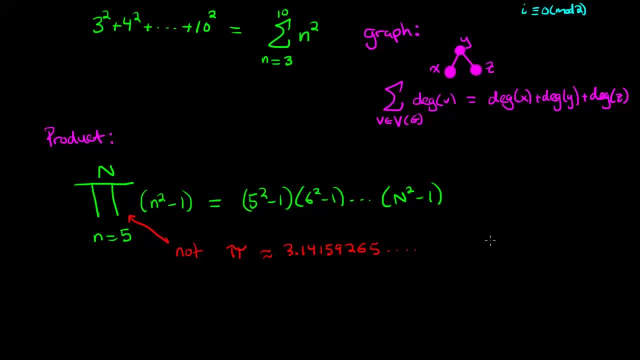 3.15.. 4159265, etc. Notice that we can also use this notation to define n factorial, like we did at the beginning of the video, and factorial is now the product of i, for i equal 1 up to n, So we get 1 times 2 times 3, all the way up. 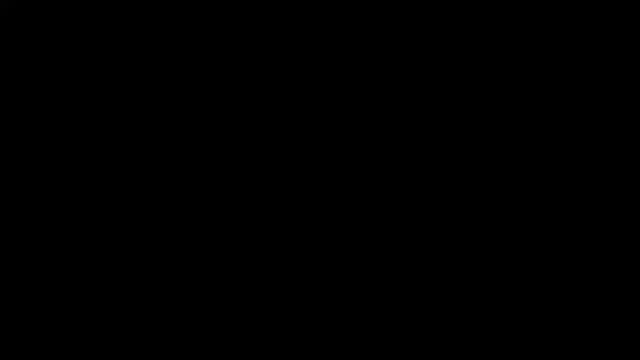 to n minus 1 times n. The last bits of notation that I want to show you deal with quantifiers. Probably the most important quantifiers is backwards e, which means there exists, And upside down a, which means for all. If we think about a little example, we could 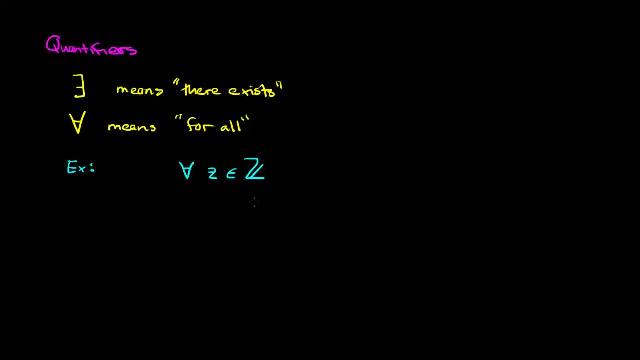 say something like: for all little z in capital Zed- which, by the way, this means the set of all integers- There exists little zed prime in capital Zed, such that Zed prime is bigger than Zed. This is a true statement, because for any integer, 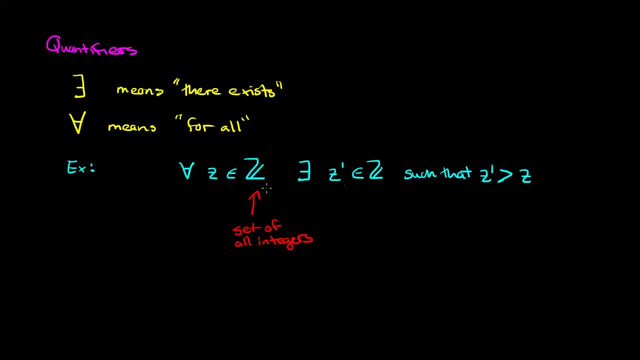 that you pick, you can always find a bigger one. If you want to just add one to the one you picked, found a bigger one. Okay, quantifiers are fun, but let's conclude with a tiny bit of logic. This symbol here means if and only if. and this symbol with only one directional arrow means 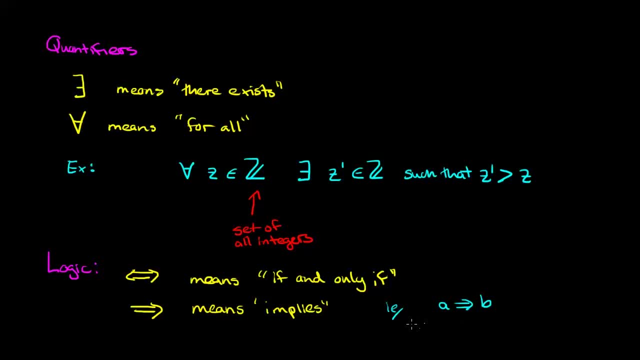 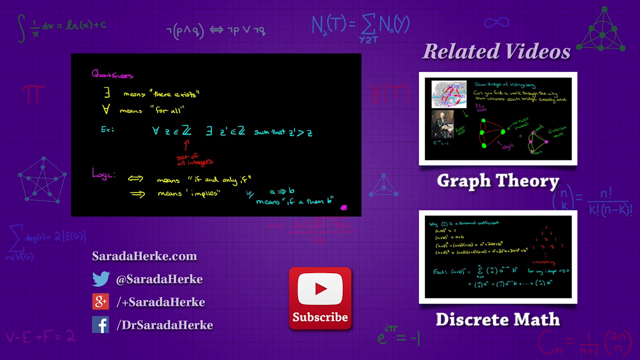 implies. For example, A implies B is the same thing as writing if A, then B. And last but not least, perhaps one of my favorite symbols is the little square that you put at the end of a proof. So I hope you've enjoyed this brief introduction and quick introduction. to lots of mathematical notation. I'll see you next time. 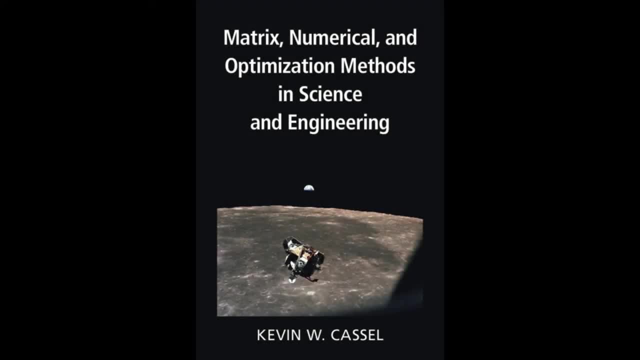 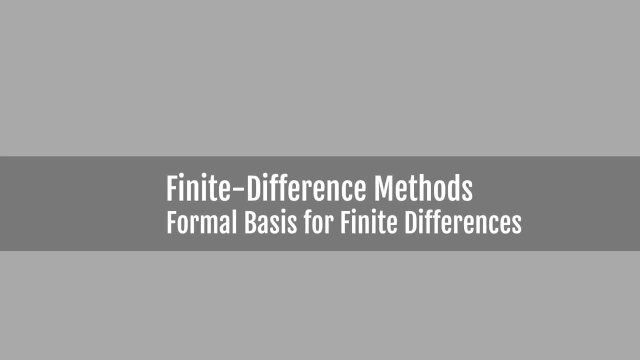 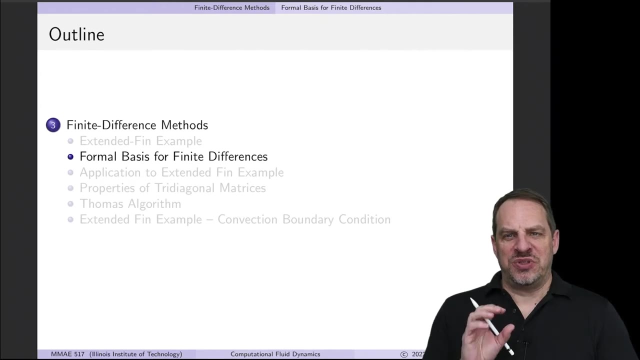 In the previous video we considered the extended fin examples, So this is a specific physical problem. In order to introduce the first two steps of the numerical solution procedure and to see where we need these finite difference methods, we got a second order: ordinary differential. 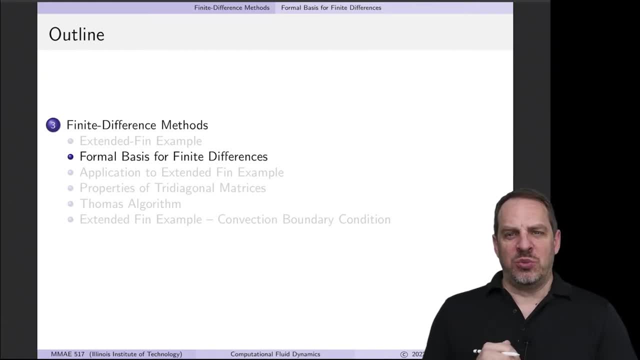 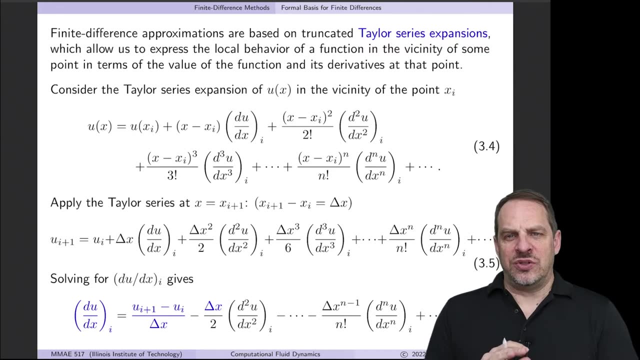 equation that we need to solve, And in this video we're going to look at the formal basis for finite difference methods. These are based on Taylor series expansions, So I'll show you how that's utilized to get the approximations that we intuitively obtained in the previous. 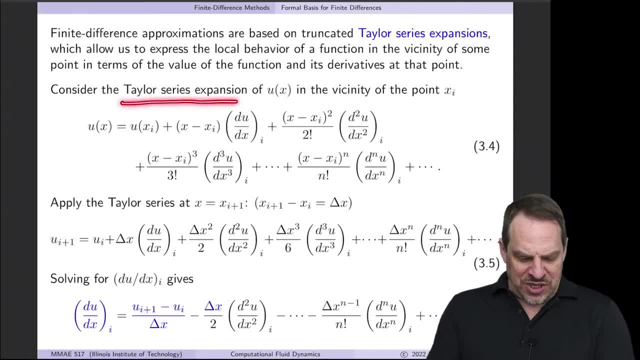 video. So let me remind you what the Taylor series expansion looks like. So our dependent variable here is u. u is a function of x, And what we're doing is we're looking at the solution at a point x which is close to a point x sub i. So I want to know u at that value of x, And so it's. 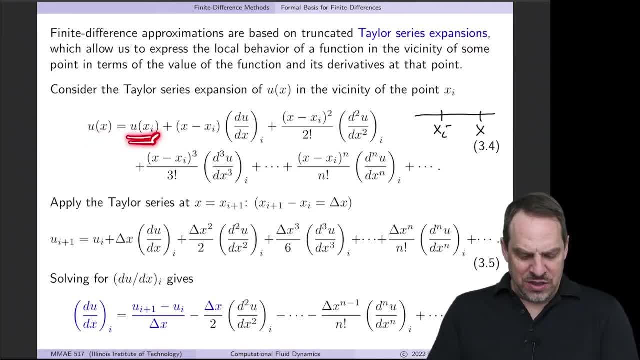 equal to the u at the close by value u at x sub i. plus these terms, Each term has a derivative in it: du dx d squared, u dx d cubed, u dx cubed, and so forth, all of which 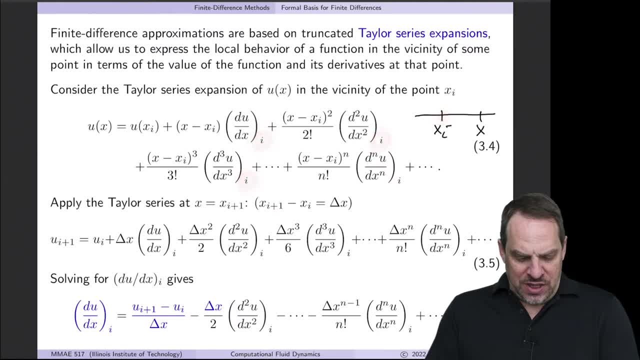 are evaluated at this point, And then we have the distance from the point, the distance from x to xi and so forth, squared, cubed, And if you include all of the terms in this expansion, you get an exact representation of the function in terms of information. just at that point It's pretty remarkable when 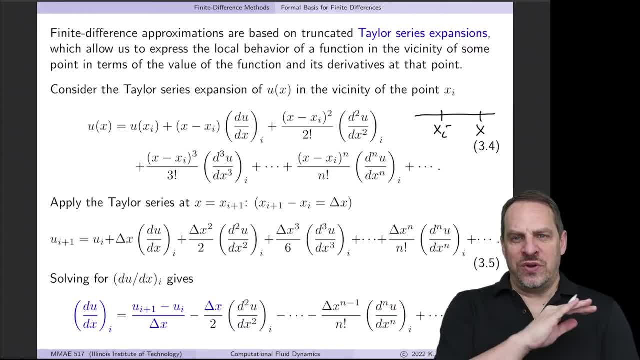 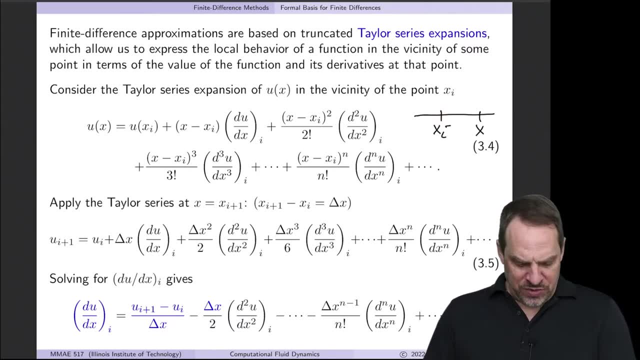 you think about that, You can know all there is to know about an entire function u of x just by knowing information about derivatives at a particular point. That's pretty remarkable. Now, the way we apply this is: we're going to take our Taylor series, we're going to apply.